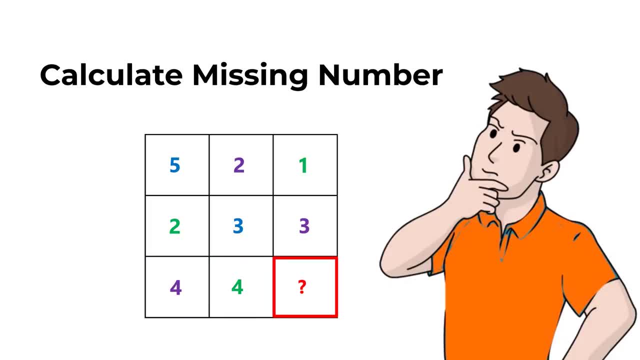 one number is missing. This is the one that you need to calculate. Once you complete the calculation, you need to select one of the four different choices: Choice A – 0,. choice B – 1, choice C – 2 and choice D – 3.. 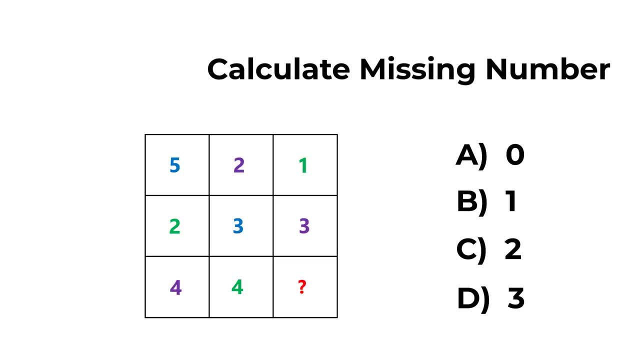 Take a look closely and see if you can identify the missing number. Give yourself 5 to 10 seconds- maybe 10 to 15 seconds, to see if you can come up with the right solution. Do you see the answer? Let's continue to see how we can solve this challenge and get to the correct solution together. 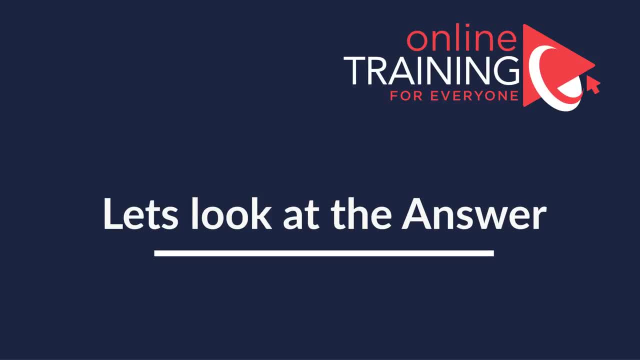 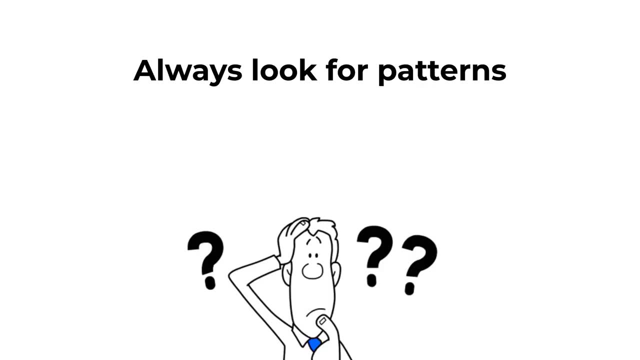 Be sure to subscribe to our channel so that you don't miss any of our videos. As usual, my advice to you – always look for patterns. In this particular case, we need to look at the patterns inside the Rows and then inside the Columns. Let's look at the 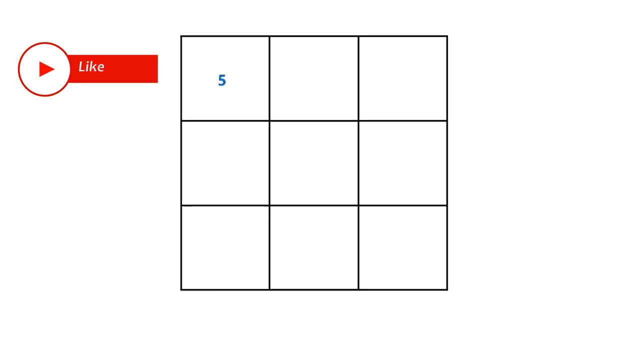 first two rows to see if we can get a pattern. The sum of 5 plus 2 plus 1 equals to 8.. The sum of 2 plus 3 plus 3 also equals to 8.. So there might be a pattern. Let's look if there is a. 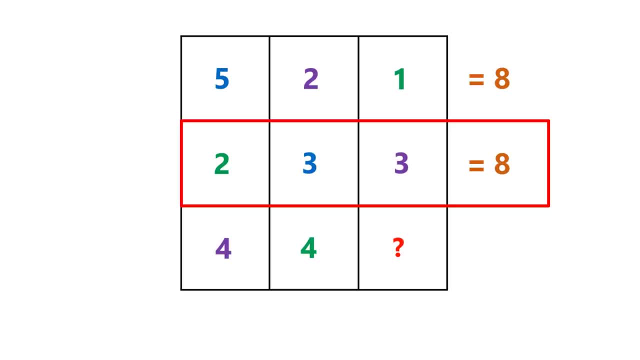 pattern for the columns that have full sets of numbers equals 11.. 2 plus 3 plus 4 equals 9, so there is no pattern In this case. we can relatively simply use the pattern from the rows. This would allow us to calculate the third row. 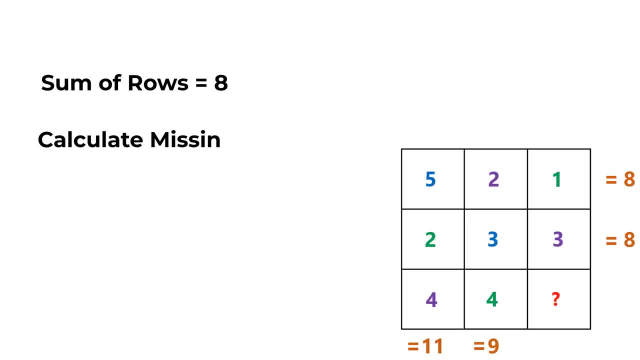 If we know that the sum should be 8, we can assume that the 4 plus 4 plus question mark, which would be representing the missing number, would be equal to 8, so the missing number would be equal to 0.. The correct choice here is choice A, 0.. Hopefully you've nailed this. 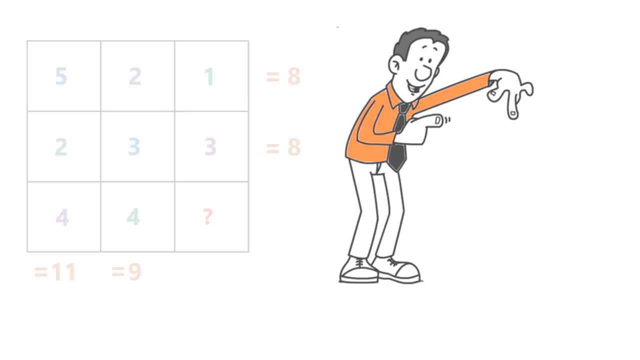 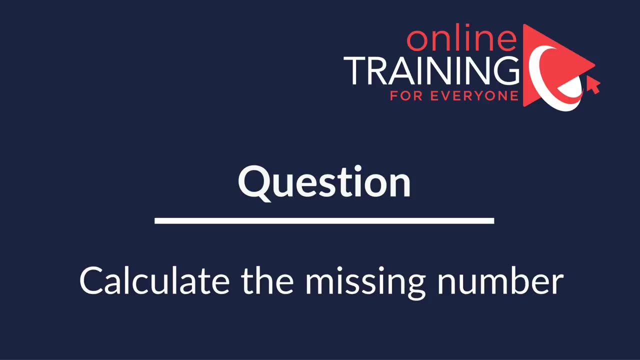 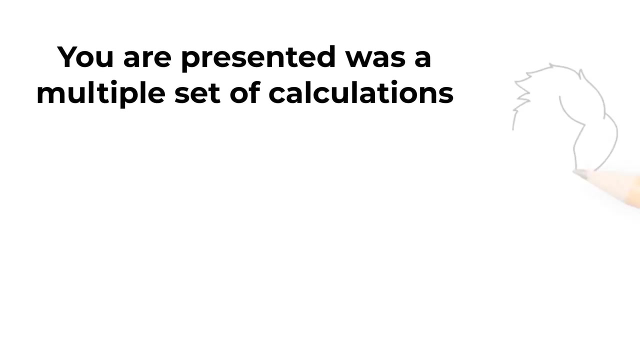 question on your own and now know how to answer similar problems on the test. You're going to love this problem because it is so confusing. You're presented with multiple set of calculations. In our case, we have two full calculations and one calculation. 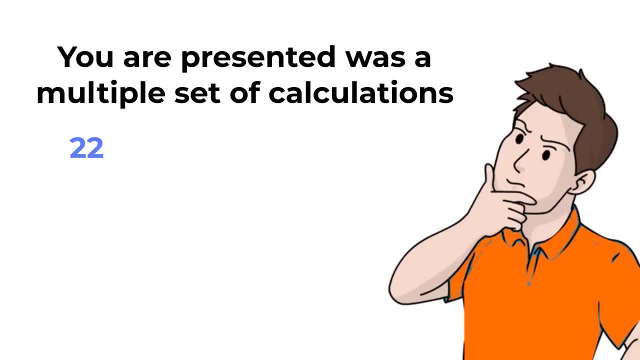 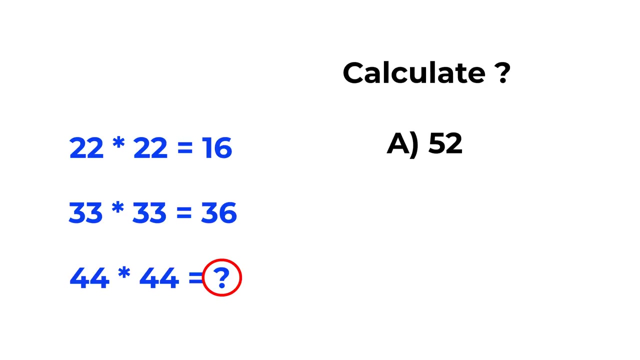 is missing the final value. The first calculation is: 22 multiplied by 22 equals 16.. Second calculation is 33 multiplied by 30.. The last calculation is 44 multiplied by 44 equals question mark, and you need to calculate question mark. You have four different choices: Choice A: 52.. Choice B: 56.. Choice C: 60.. 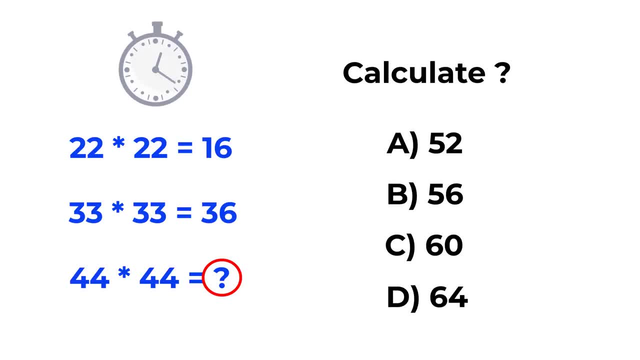 And choice D 64.. Do you see the answer? It's not obvious. so give yourself 5 to 10 seconds, maybe 10 to 20 seconds, to see if you can come up with the solution. I'm going to reveal the answer and we're going to get to the correct solution together. 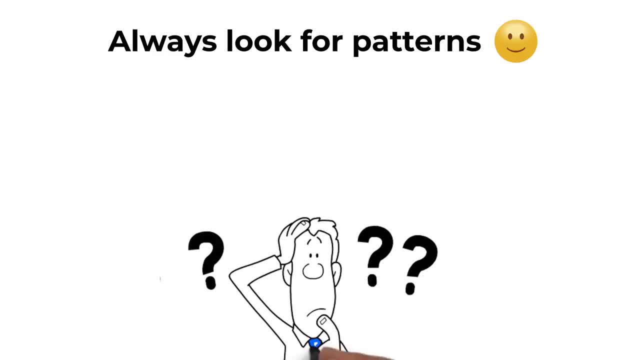 Typically to solve these types of problems, you need to identify the pattern And in this particular case, the pattern is that the sign and parentheses are hidden in between digits and are not presented on the screen. Let's look at the first two examples: 22 multiplied by 22 equals 16.. It is 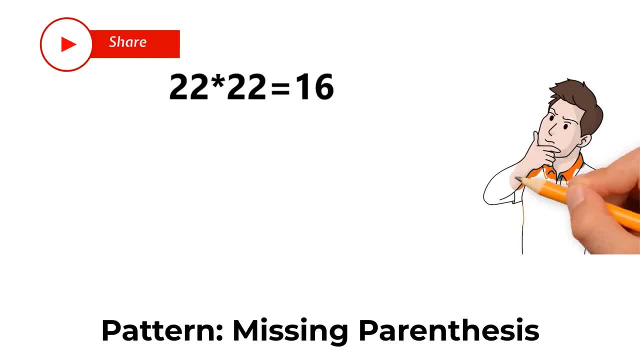 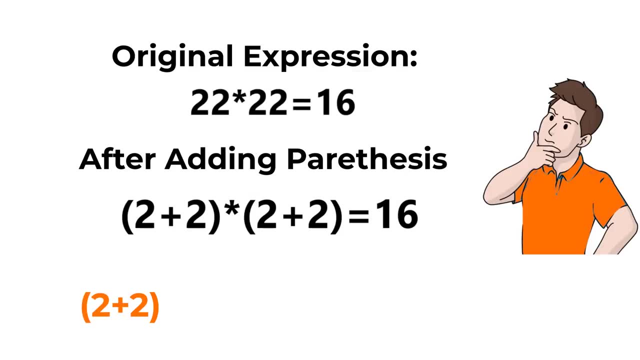 not so obvious because it doesn't go along with the rules of conventional math, But if you add parentheses and in parentheses add 2 plus 2, multiplied another set in parentheses, 1 plus 2, you will be multiplying 4 by 4, and the result will be 16.. Same thing with 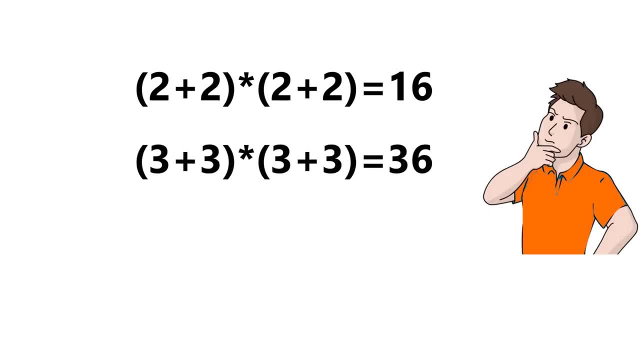 3 by 3.. If you add in parentheses 3 plus 2, multiplied by another set in parentheses 3 plus 2, e census 6 plus 6, you will be multiplying fifty-sixpauses by fifty-sixpauses and the result will be 36.. Ok, so the correct answer is… 36.. So we have 6 plus 6. that equals 66. That's how we write this result. So that means we get the correct answer for the word 36.. So we can. 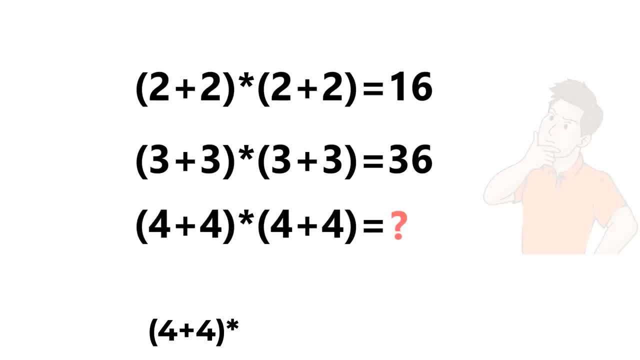 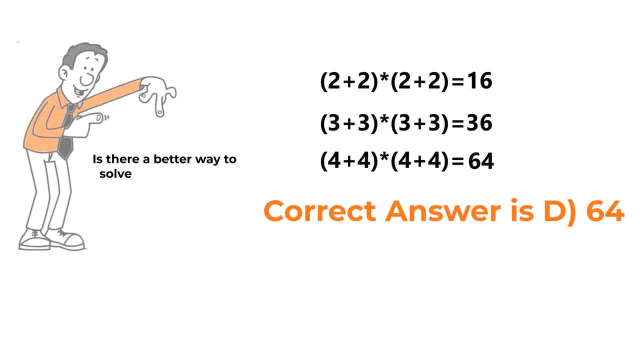 answer here is the set in parentheses 4 plus 4 multiplied by another set in parentheses 4 plus 4, which would be multiplication of 8 by 8, and the end result of this would be 64.. so the correct answer here is choice d, 64.. hopefully you've nailed this question and now know how to answer. 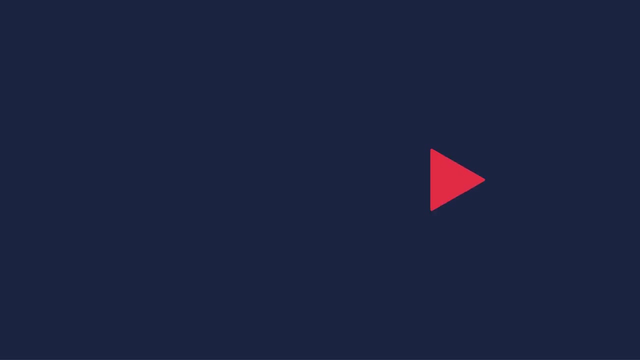 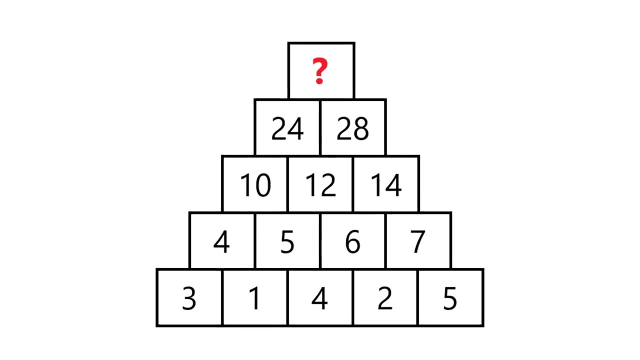 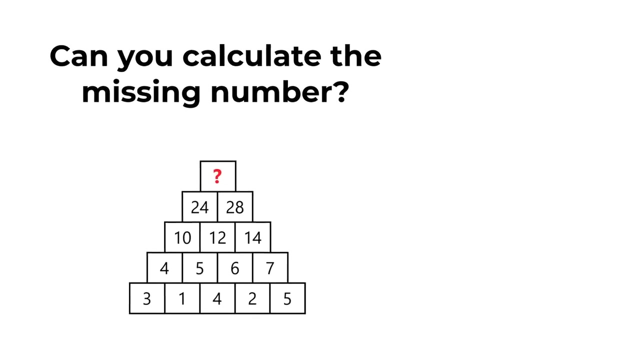 similar problems on the test. here's one of my favorite questions, and it is my favorite because it is so unusual. you are presented with the pyramid. pyramid contains five different layers. if we go from the top to bottom, you have a question mark. this is the number that you 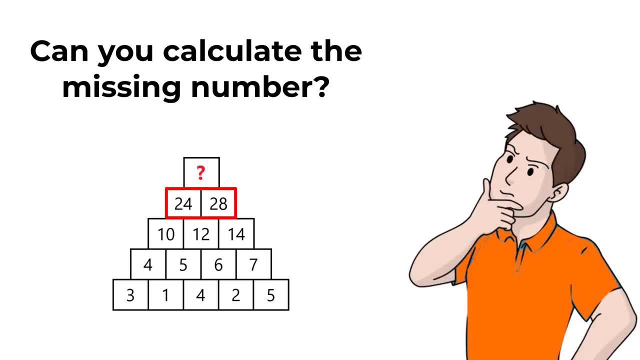 need to uncover. the next layer contains numbers 24 and 28. layer below this contains numbers 10, 12 and 14.. next layer has 4, 5, 6 and 7, and the last layer has numbers 3, 1, 4, 2 and 5. 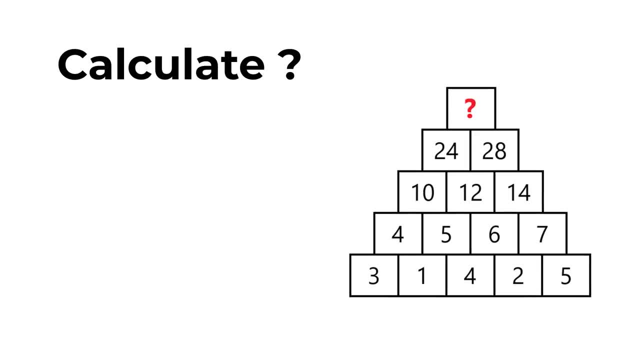 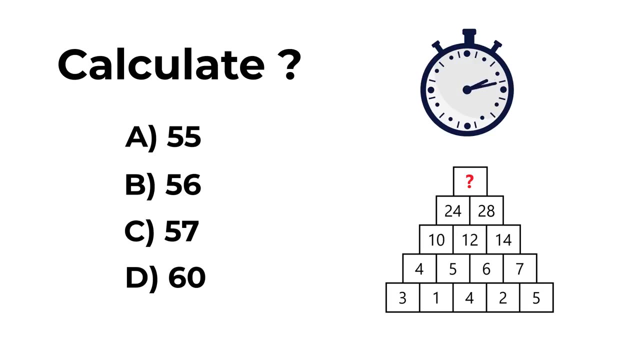 you're presented with four different choices for the missing number: choice a: 55, choice b: 56, choice c: 57 and choice d 16.. do you see the answer? you will be surprised how simple it is to get to the answer when we go to the next step. give yourself 5, 10, maybe 15 seconds to see if you can calculate. 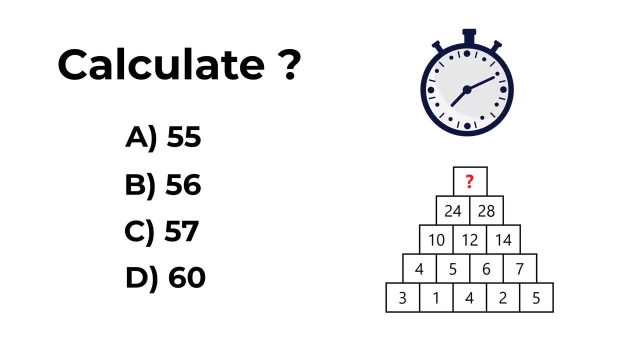 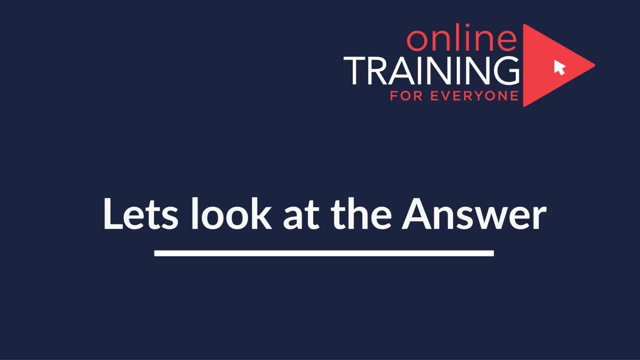 and get to the correct answer. did you figure it out? let's continue and see how we can get to the correct solution together. let's continue and see how we can get to the correct solution together. well, here, to be honest, i try to trick you. i went in describing numbers from top to bottom, but in 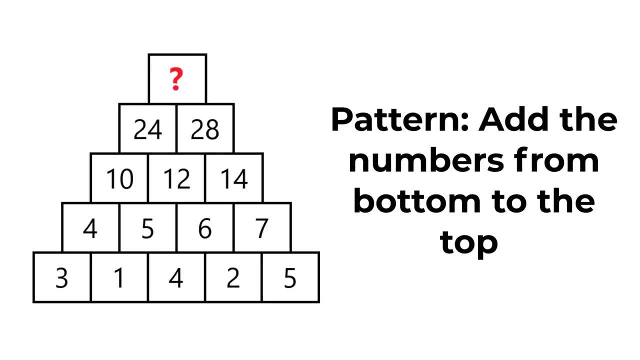 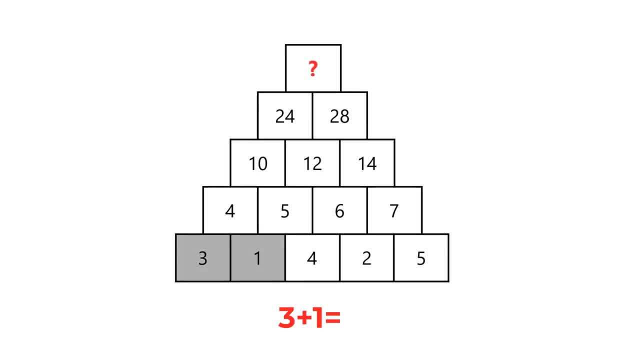 reality you should be looking at the numbers from bottom to the top. if we start from the bottom row, for example with numbers three and one, you see that the sum of three and one will add up to four. but then it gets trickier if we go from the second row to the third row. 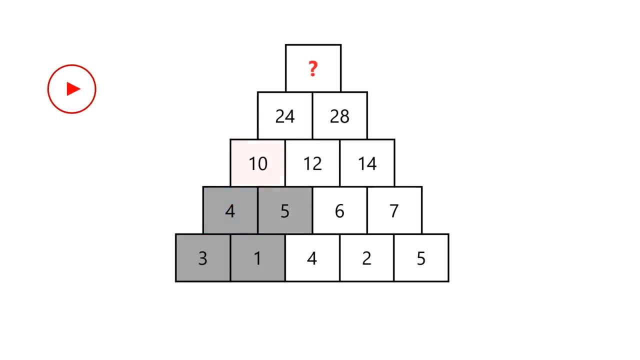 you see that the four and five does not necessarily add up in ten. four and five adds up in nine, and then you need to increment it by one. if you go to the next layer, you need to increment it by two and then, in the final row, you need to increment it by three. so the correct answer here. 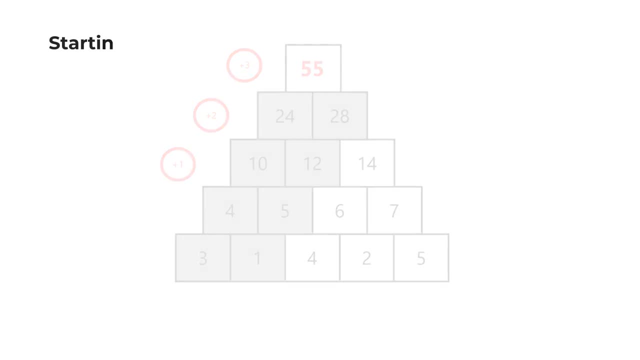 is choice 55.. let's recap: starting with the bottom row, the sum of two squares results in the number in the next row. for example, 2 plus 5 equals 7.. however, as each level continues, the sum increases by 1.. you did increase your number 7 twice when youiro repeated its steps, one by one to each level. 6 does not change. so you have Теперь 2, 3, two x 6, c. face the other side of the value, 9, and you do not finished a number again. increase it: e, the lenght of the value more higher than 1 plus 5. you have the last cell, number 3, the number gain, UM. on each level 5. you increase Nada on each level 55. so let's recap. starting with the bottom row, the sum of two squares results in the number in the next row. for example, two plus 5 equals 7. however, as each level continues, 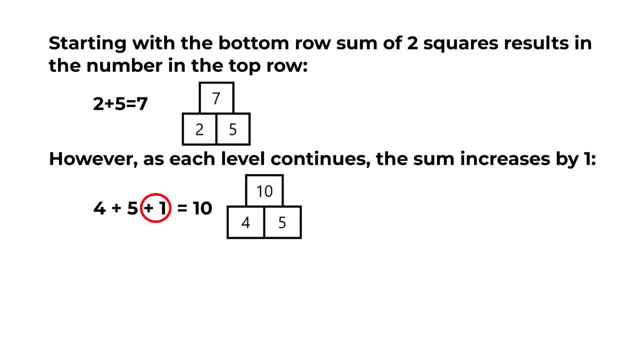 4 plus 5.. We need to increment and add 1 to get to 10.. So the answer is calculated by adding up 24 plus 28 plus 3, which would be equal to 52 plus 3 and would be equal to 55.. The correct answer. 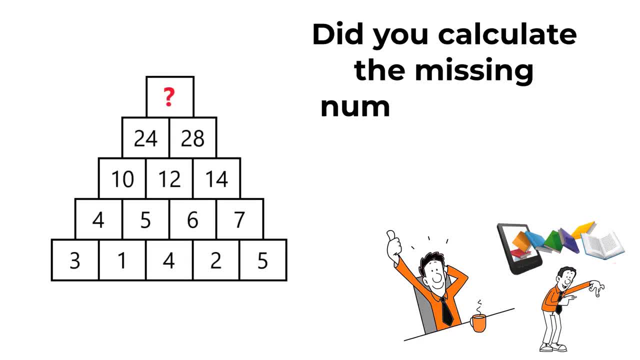 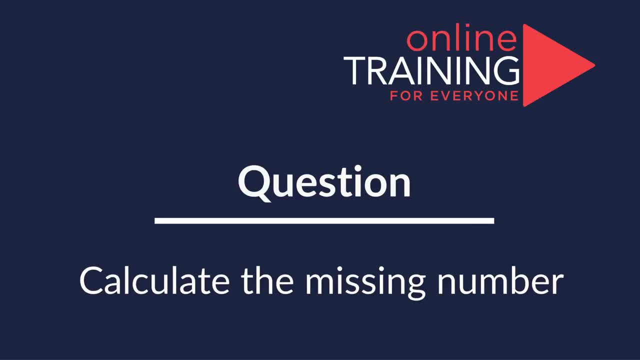 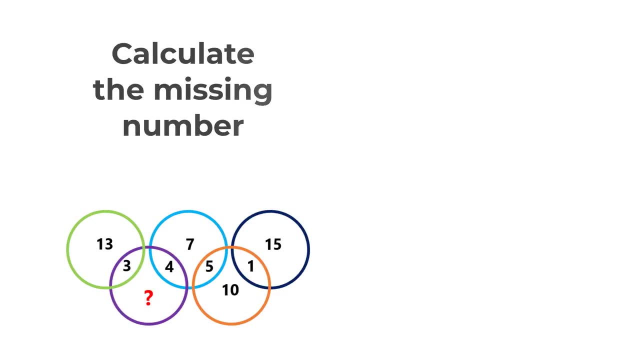 here is choice A 55.. Hopefully you've nailed this question and now know how to answer similar problems on the test. This is one of my favorite questions because it is very frequently used in the test. You're presented with five crossing circles. All circles are of the different colors. 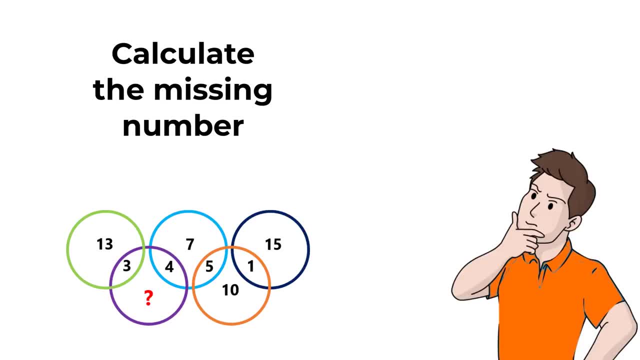 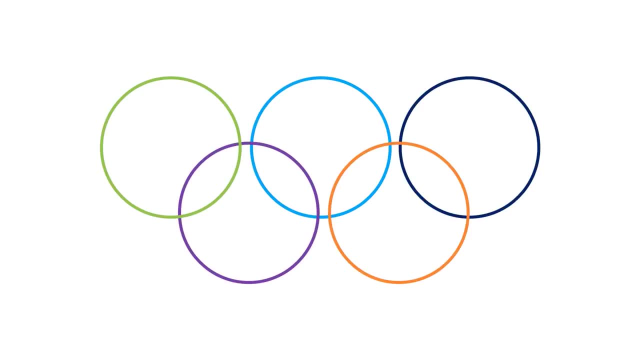 There are numbers inside the circles as well as the numbers on the intersections of the circles. In this particular case, you're presented with five different circles, all of them different colors, and the numbers that you see on the screen are 13.. 3,, 4,, 7,, 5,, 10,, 1, and 15.. There is also one number missing, which is highlighted with the. 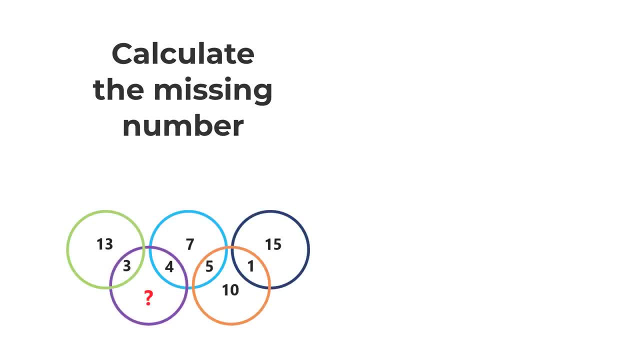 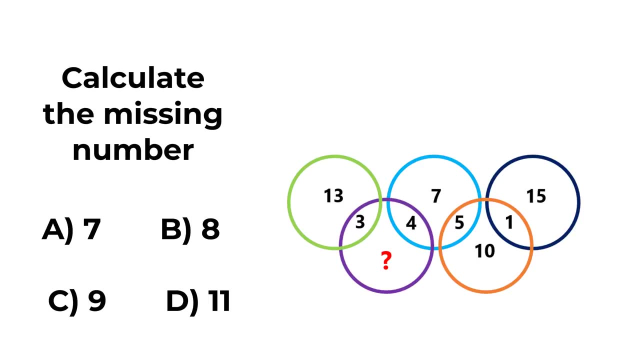 question mark. You need to calculate the missing number and the choices are choice A- 7,, choice B- 8,, choice C- 9, and choice D- 11.. Give yourself a few seconds, maybe 10 to 15 seconds. This is about 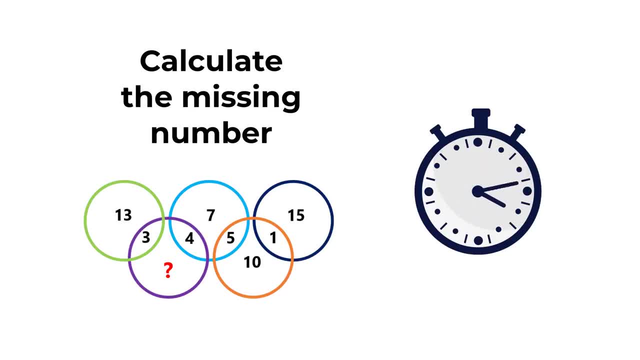 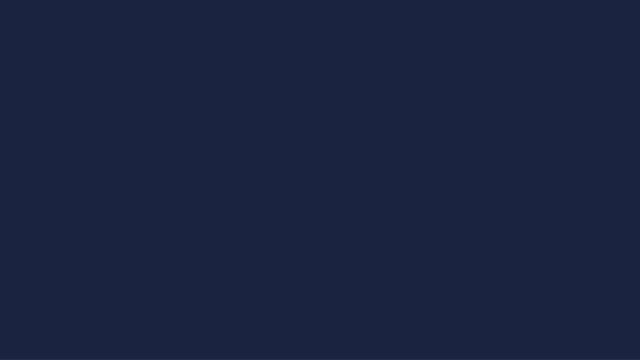 as much time as you get on a typical test to calculate the answer. Do you see the solution? Let's continue To see how we can get to the correct solution and solve this challenge together. As you might have figured out by now, sum of each numbers in the circle adds up to 16.. For example, 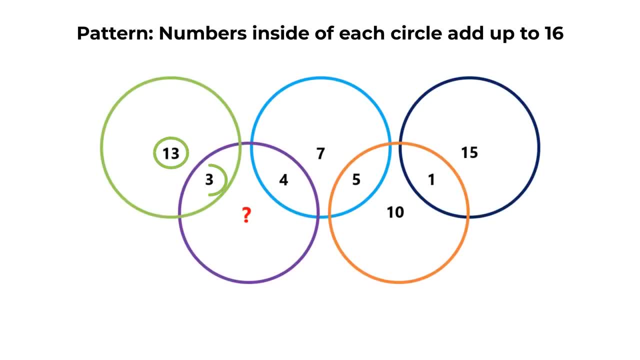 let's look at the green circle. We have numbers 13 and 3,, and 13 plus 3 equals 16.. In the blue circle, we have numbers 4 plus 7 plus 5, and all of them add up to 16.. In the black circle, 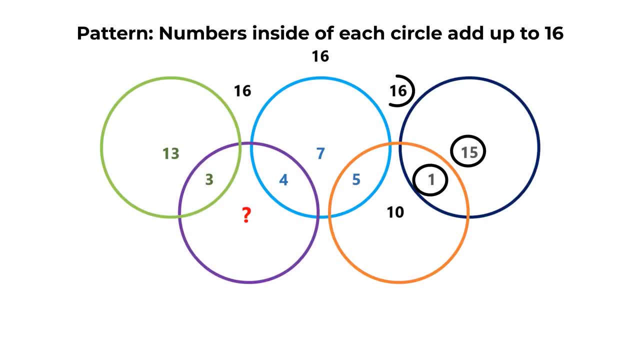 we have 1 and 15 also adds up to 16.. And in the orange circle we have 5 plus 1 plus 10 also equals 16.. So to calculate question mark, which is the missing number, we need to add 3 plus 4. 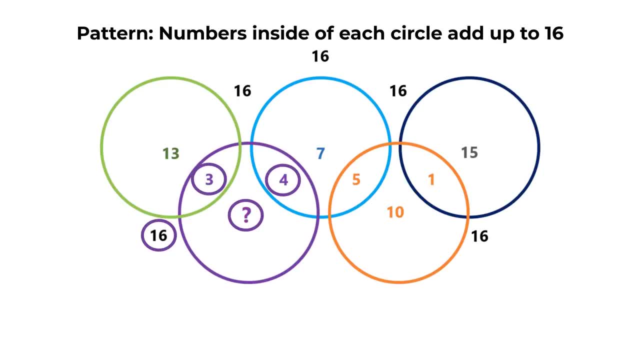 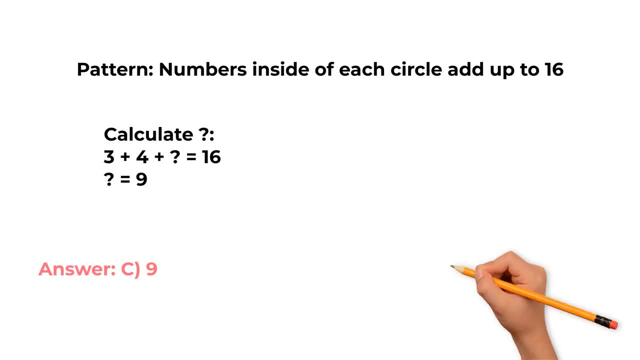 plus question mark and make an equation to make it equal 16.. After doing the calculation, you see that the question mark and the missing number equals 9.. So the correct choice here is choice C, 9.. Hopefully you've nailed this question and now know how to answer similar. 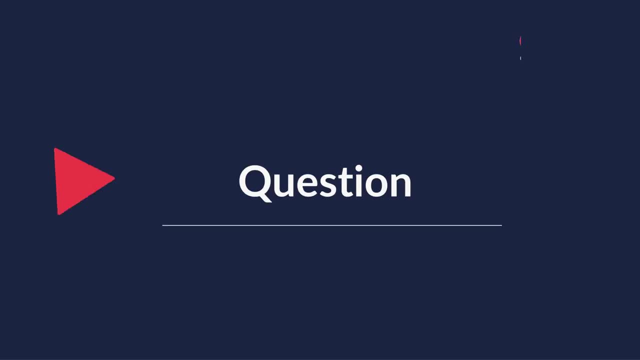 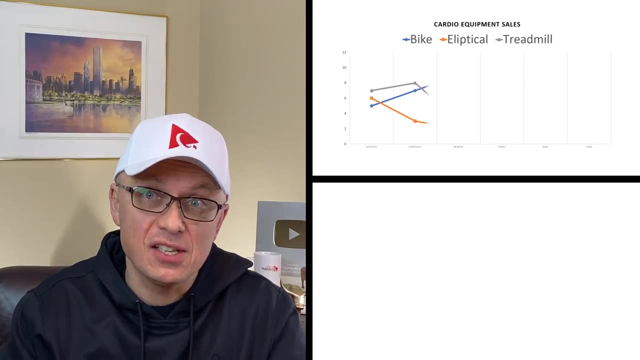 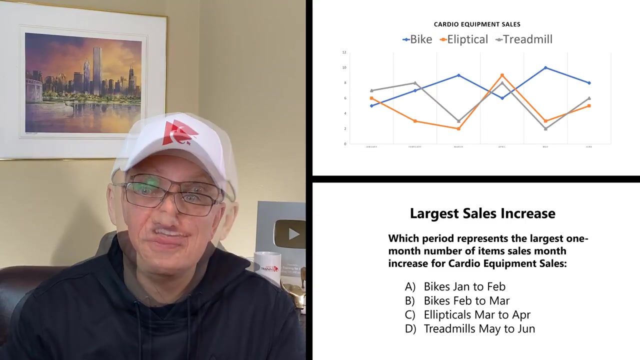 problems in the test. A lot of times you might get a question which asks you to determine the sales increase. You're typically presented with the graph which shows lines that represent different sales. In our case, we are represented with the chart that shows sales of cardio. 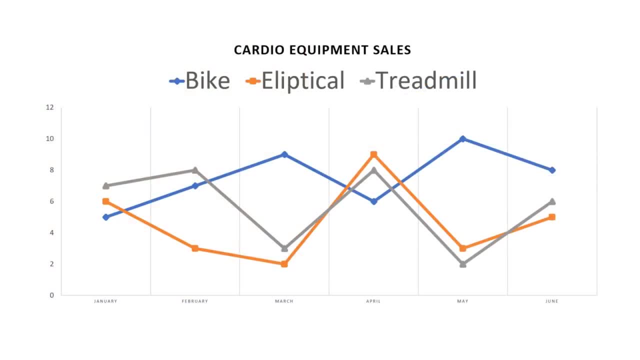 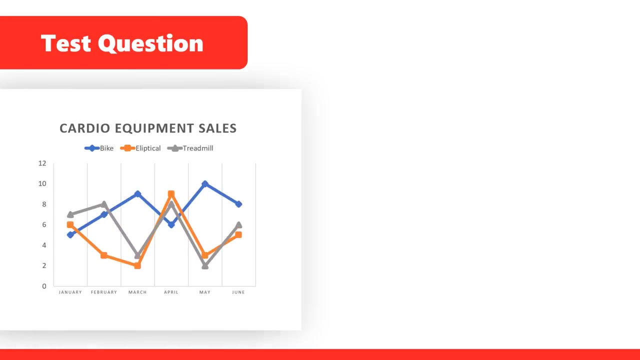 equipment. from January to June, Sales of bikes represented by the blue line, sales of elliptical represented by the orange line and sales of treadmills are represented by the gray line. The question asks you to determine largest sales increase. Specifically, you need to determine which period represents the largest. 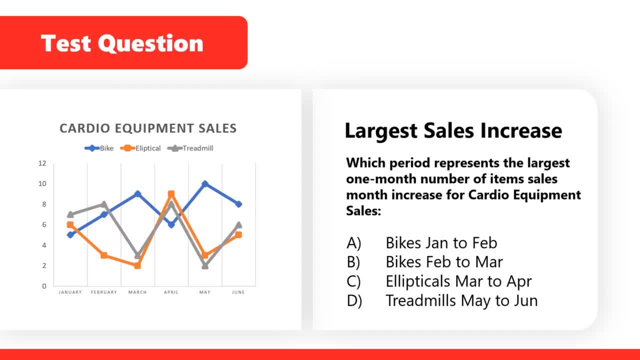 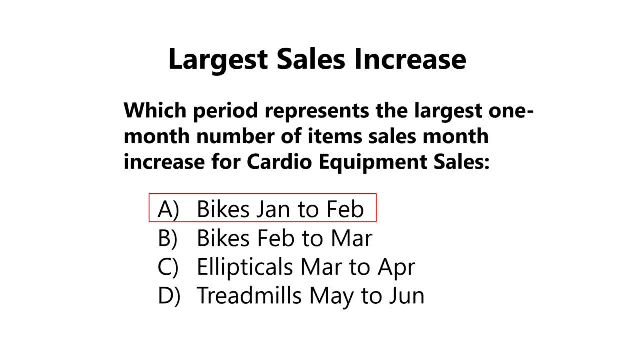 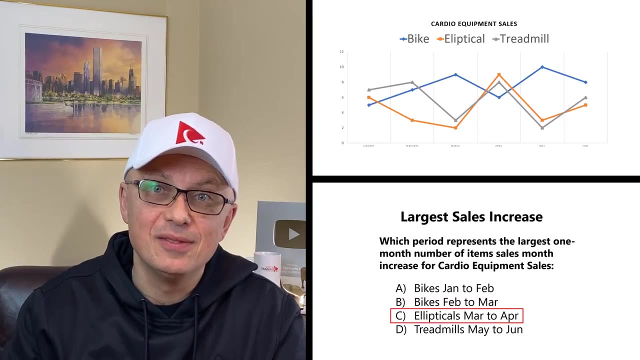 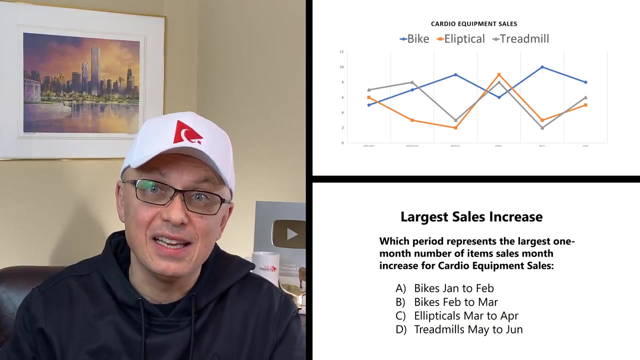 one month's number of item sales increase. for cardio equipment sales You have four different choices: Choice A- bikes- from January to February. B- bikes from February to March. Choice C- ellipticals- March to April. And choice D- treadmill made to June. Do you see the answer? You might need to look closely. 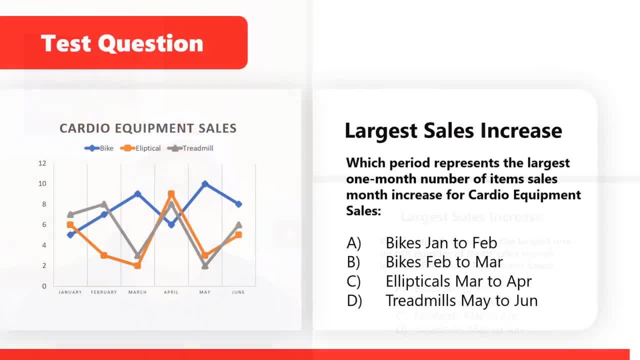 to determine the correct answer for this question. Give yourself 5 to 10 seconds to see if you can come up with the right solution. Are you ready? We're going to move forward and cover the answer for this problem and get to the solution together. 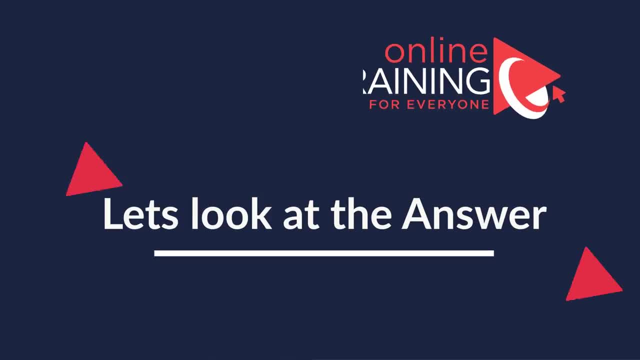 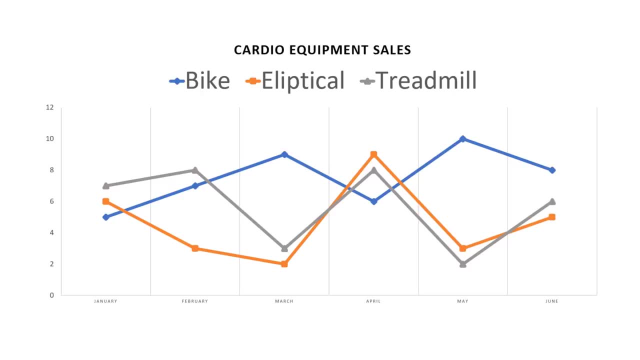 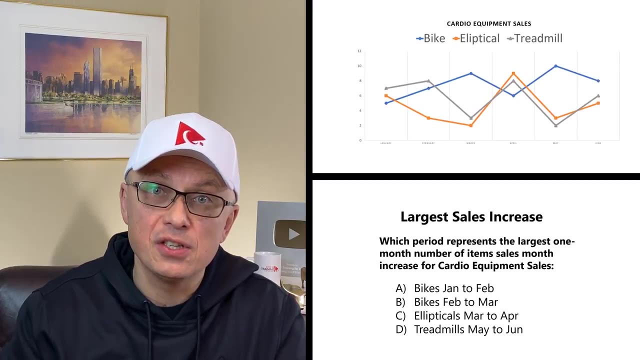 To answer this question, we need to look at the graph closely. For each data point on the graph, we need to determine the actual value And once we have all the numbers, we need to answer the question by looking at the differences for equipment sales from months to months. Specifically, 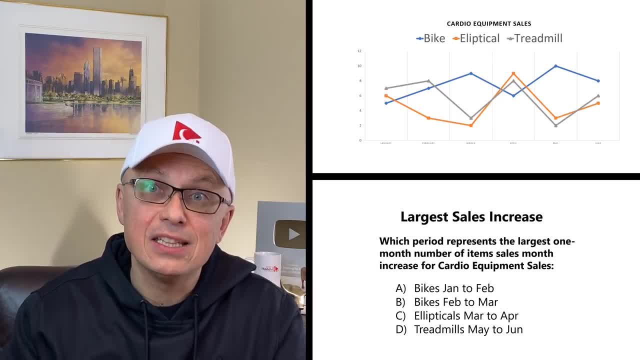 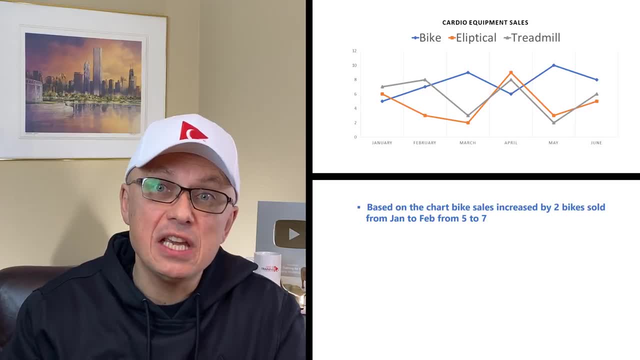 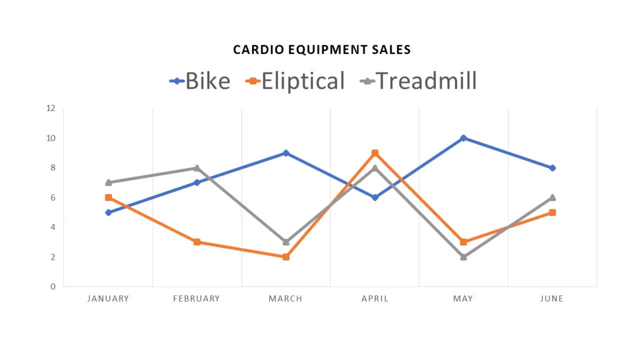 in this case, you need to evaluate four different choices that are represented by answers A through D. Let's do it together. Based on the chart, bike sales increased by 2 from January to February And the increase was from 5 to 7 items sold. Bike sales also increased by 2 from 7 to 9 between February. 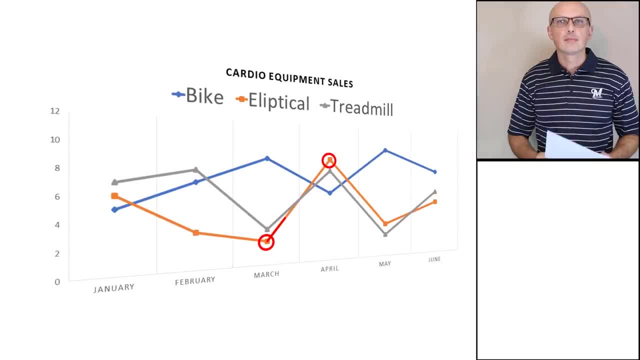 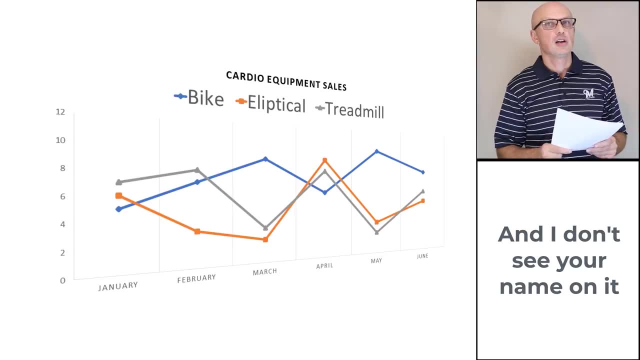 and March. Elliptical sales, on the other hand, increased by 7 from March to April, jumping from 2 to 9.. And treadmill sales increased by 4 between May and June, going up from 2 to 6.. 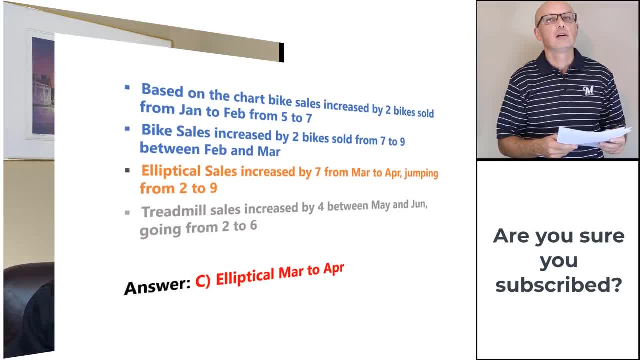 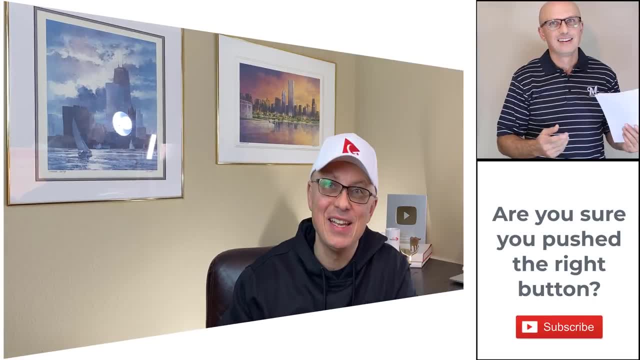 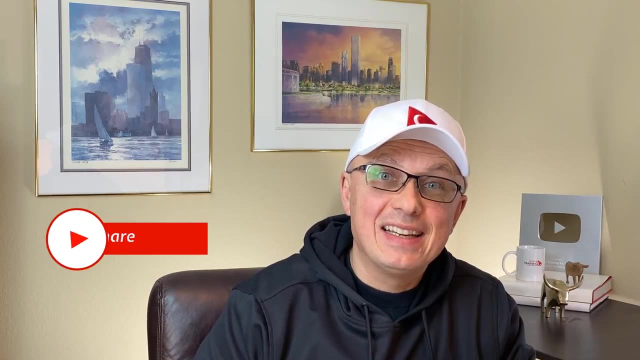 The correct answer here is choice C: elliptical sales from March to April, because jump was by 7 from 2 to 9.. Hopefully you've nailed this question and now know how to answer similar problems on the test. Thanks for watching. If you liked the content, please give us a like and consider subscribing.